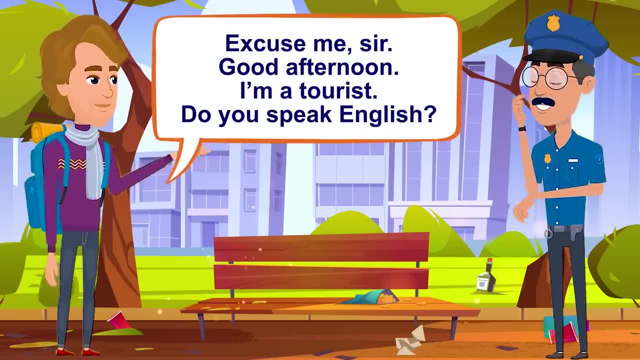 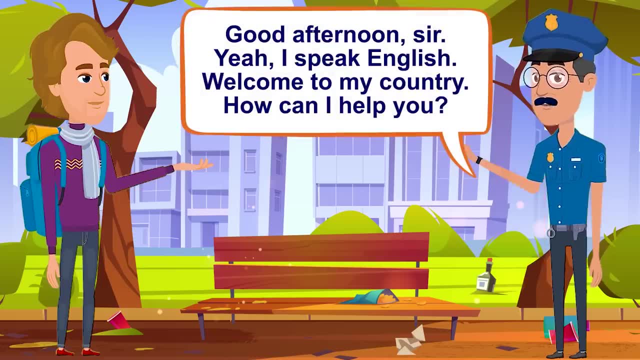 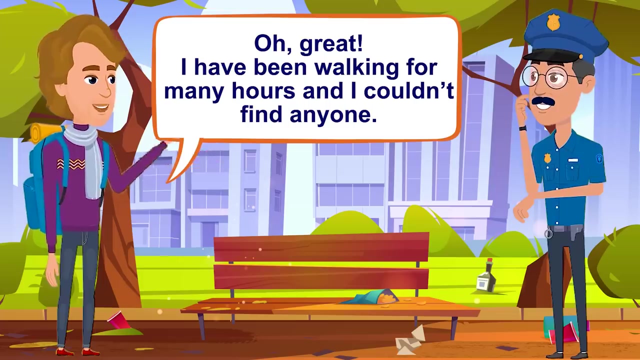 Excuse me, sir, Good afternoon, I'm a tourist. Do you speak English? Good afternoon, sir. Yeah, I speak English. Welcome to my country. How can I help you? Oh great, I have been walking for many hours and I couldn't find anyone. 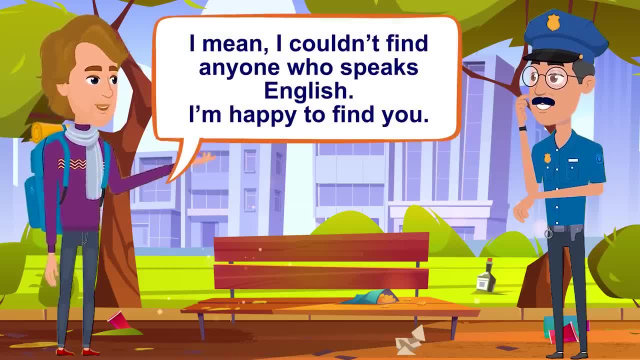 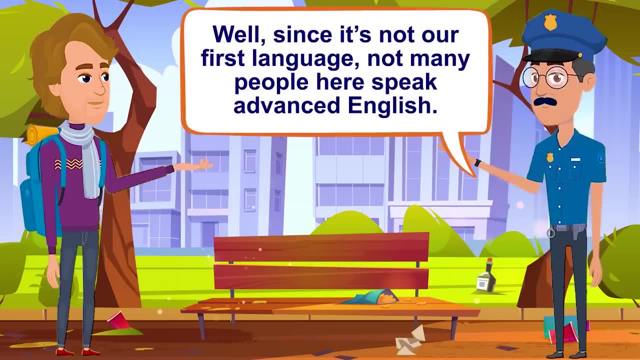 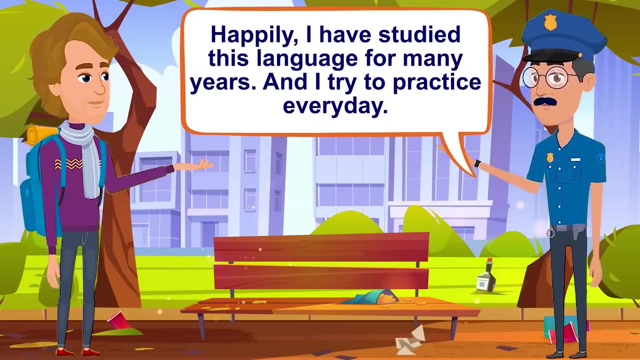 I mean, I couldn't find anyone who speaks English. I'm happy to find you. Well, since it's not our first language, not many people here speak advanced English, Happily. I have studied this language for many years and I try to practice every day. 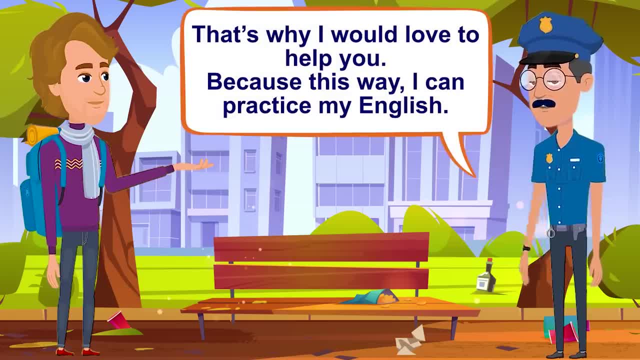 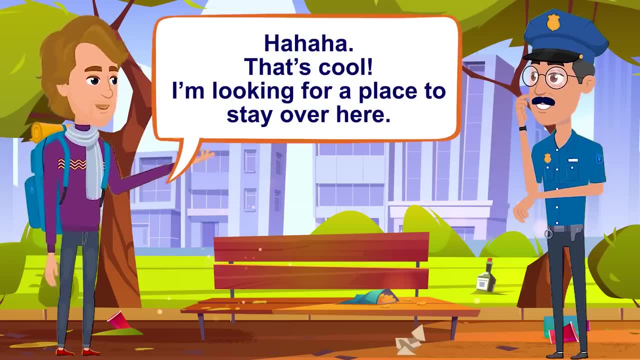 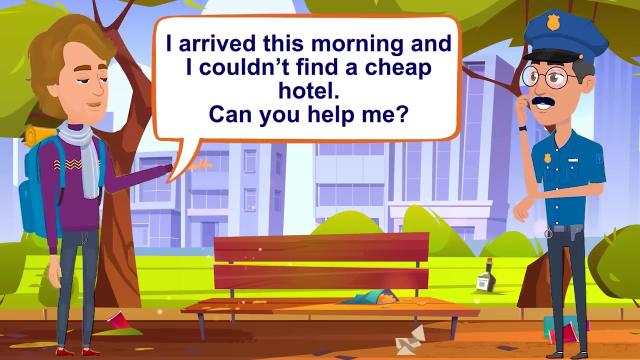 That's why I could love to help you, because this way I can practice my English. That's cool. I'm looking for a place to stay over here. I arrived this morning and I couldn't find a cheap hotel. Can you help me? 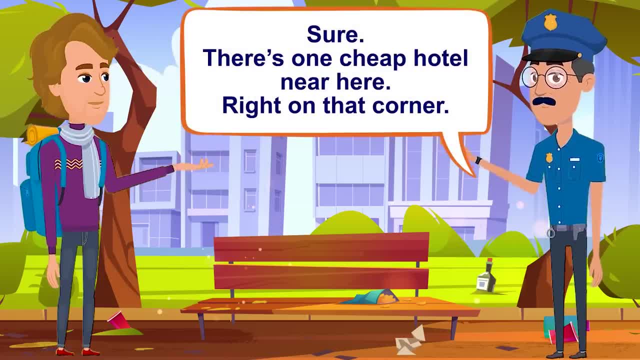 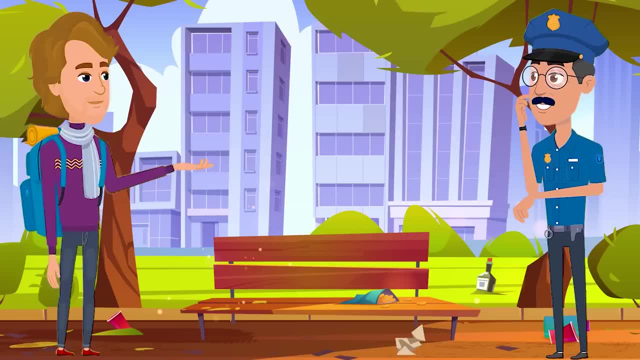 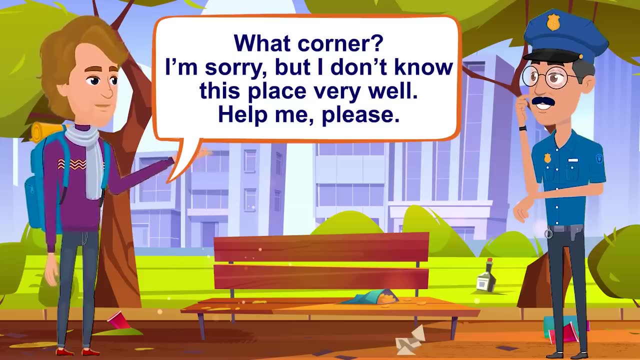 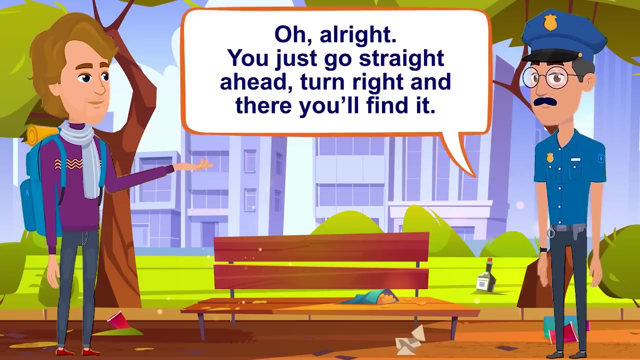 Okay, Sure, There's one cheap hotel near here, right on that corner. What corner? I'm sorry, but I don't know this place very well. Help me please. Oh, alright, You just go straight ahead, turn right and there you'll find it. 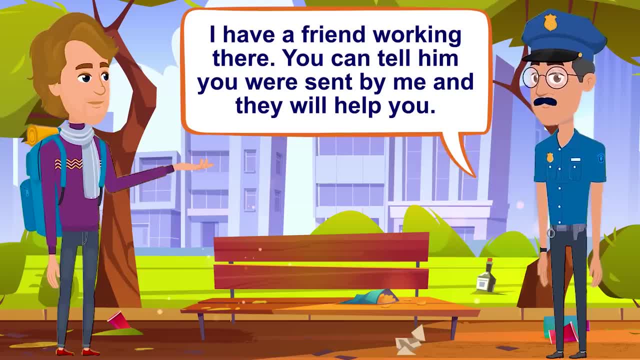 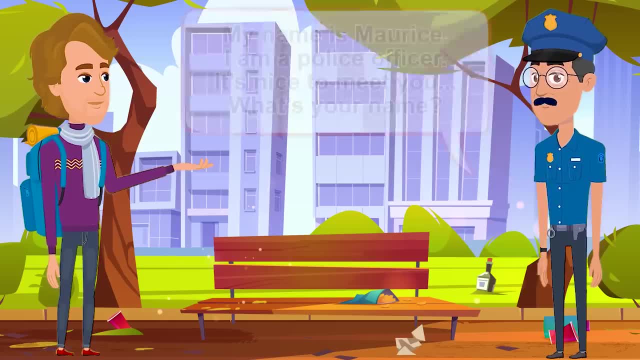 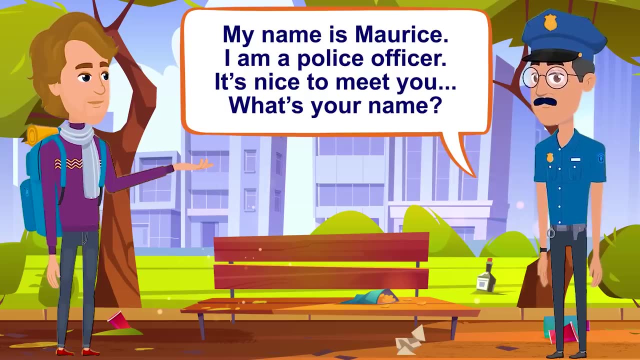 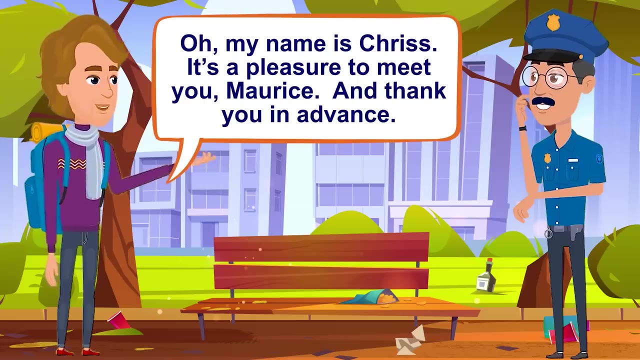 Okay, I have a friend working there. You can tell him you were sent by me and they will help you. My name is Maurice. I am a police officer. It's nice to meet you. What's your name? Oh, my name is Chris. It's a pleasure to meet you, Maurice, And thank you in advance. 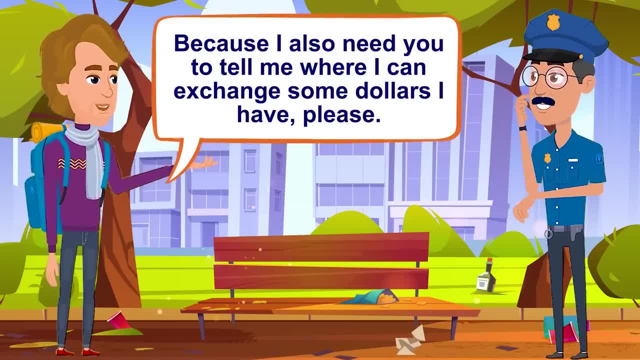 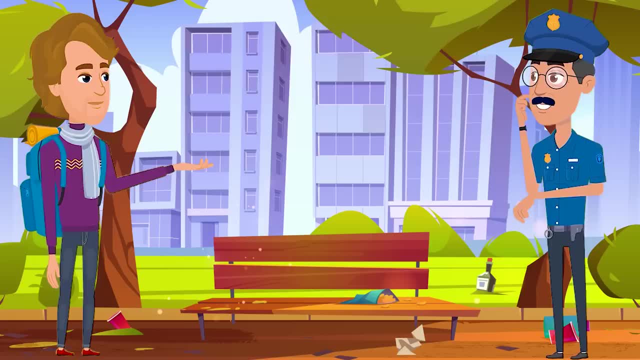 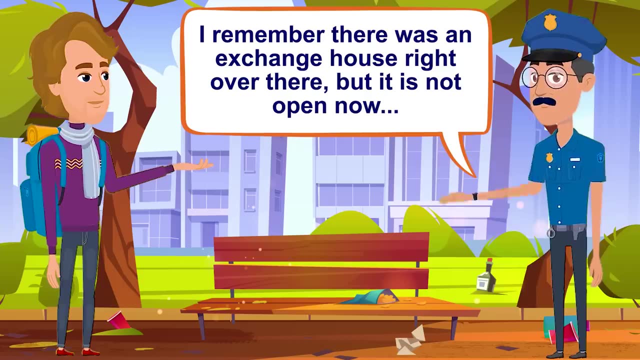 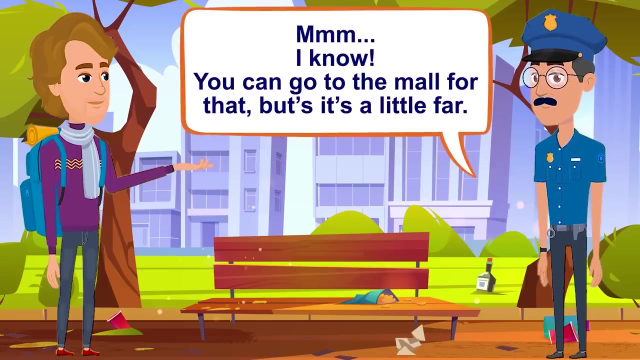 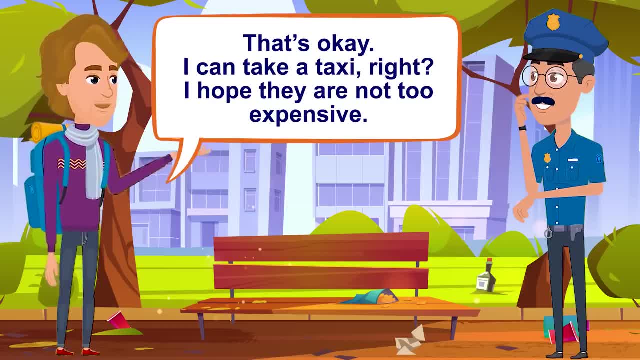 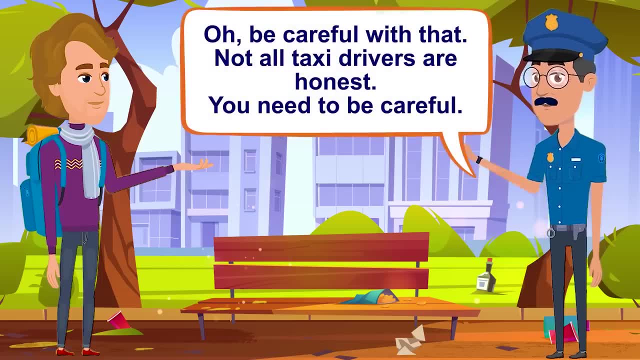 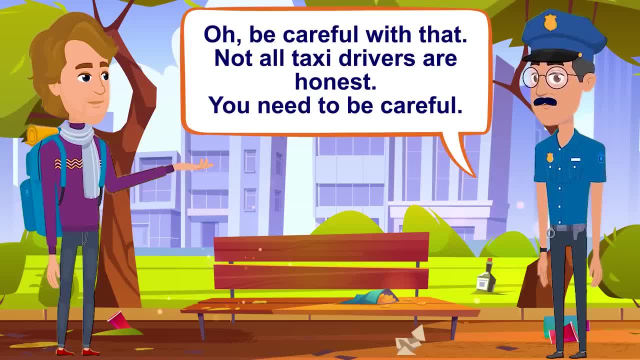 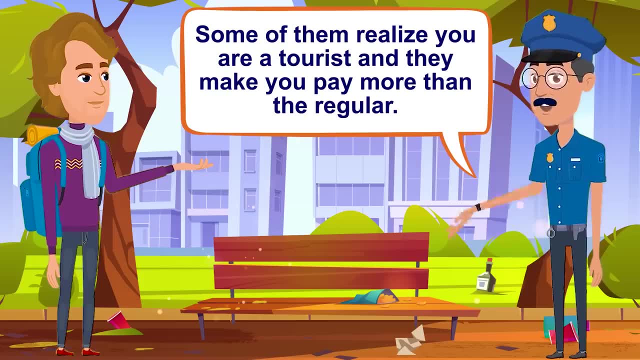 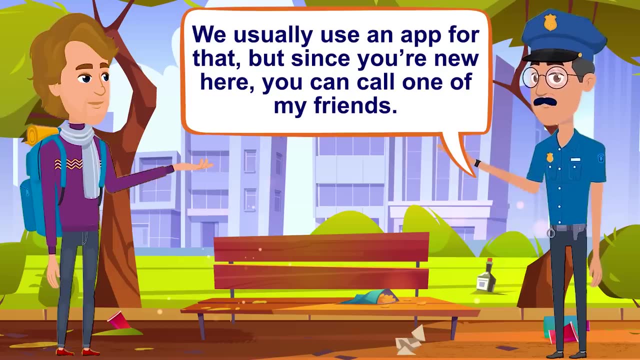 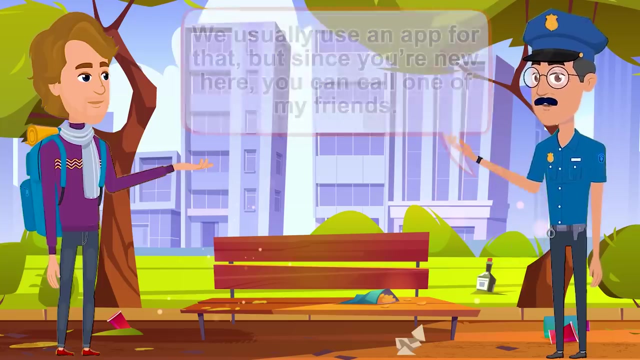 Not all taxi drivers are honest. You need to be careful. Some of them realize you are a tourist and they make you pay more than the regular Bye. I actually use an app for that, but since you're new here, you can call one of my friends. 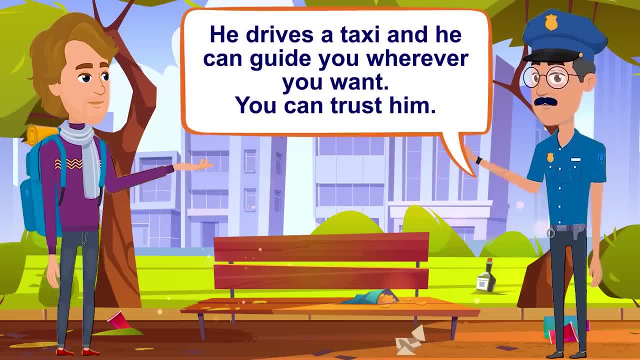 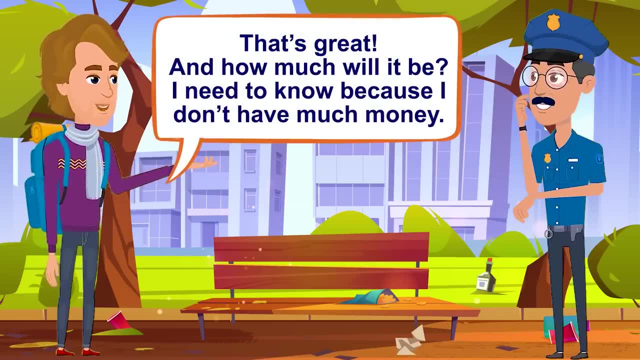 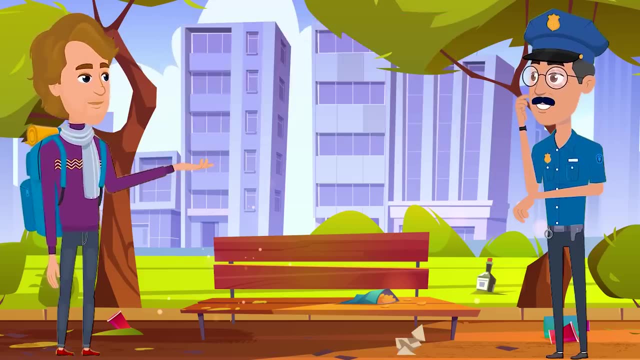 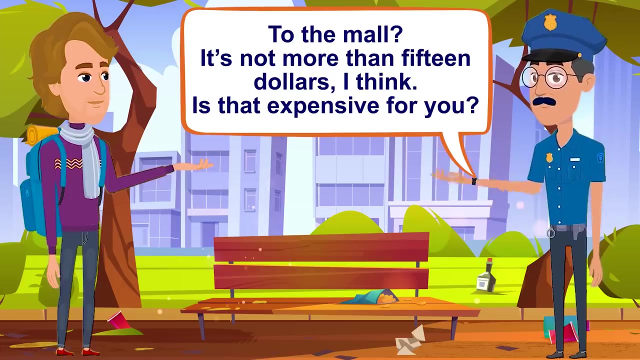 He drives a taxi and he can guide you wherever you want. You can trust him. That's great. And how much will it be? I need to know because I don't have much money To the mall. It's not more than $15,. I think It's that expensive for you. 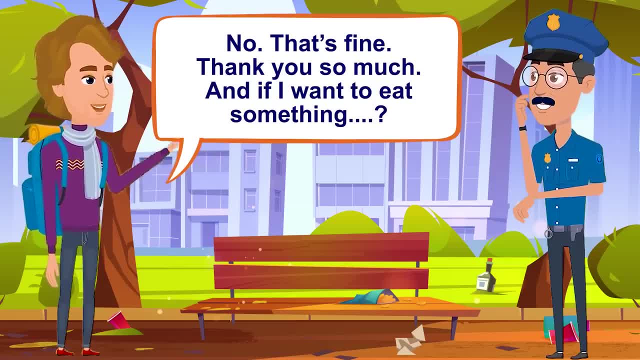 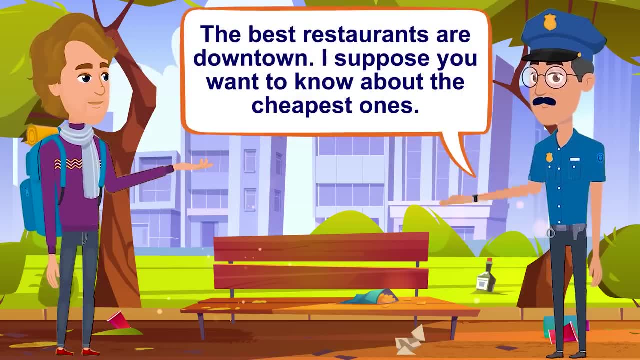 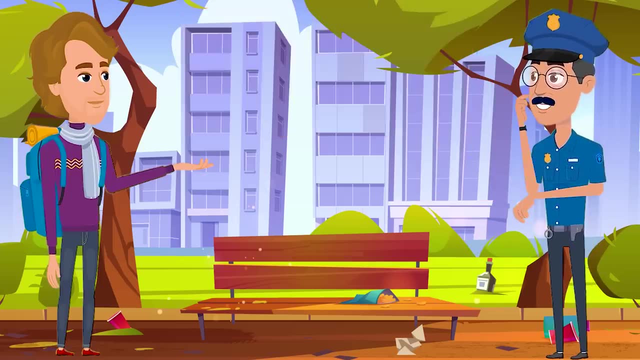 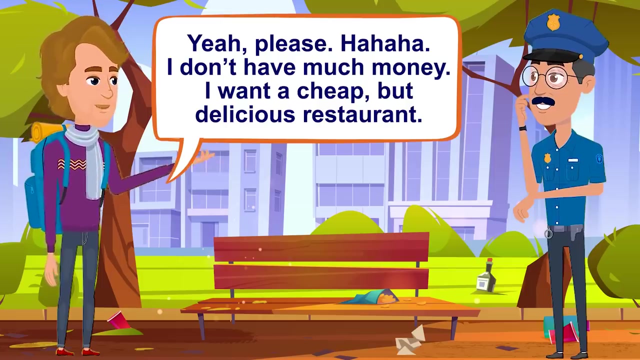 No, that's fine. Thank you so much. And if I want to eat something, The best restaurants are downtown. I suppose you want to know about the cheapest ones. Yeah, please, I don't have much money. I want the cheap but delicious restaurant. 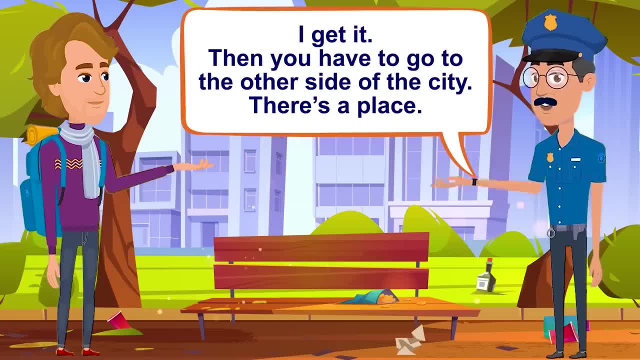 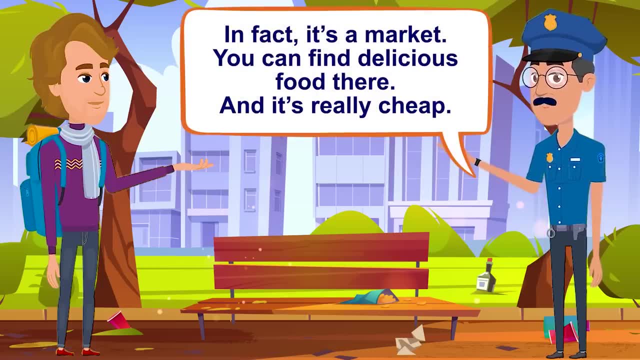 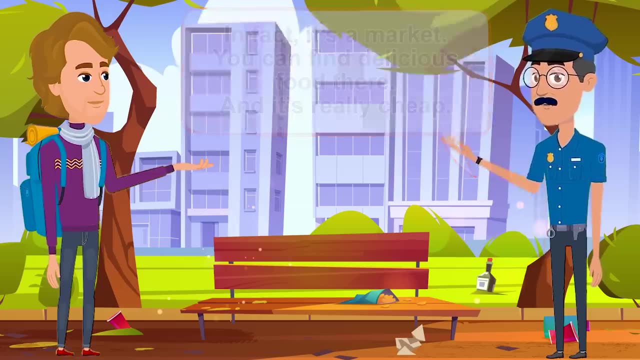 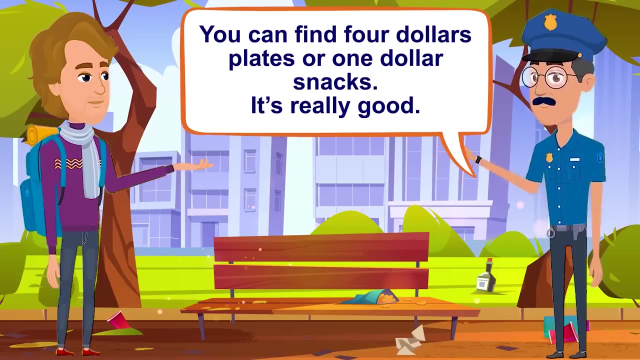 I get it. Then you have to go to the other side of the city. There's a place, In fact it's a market. You can find delicious food there and it's really cheap. You can find $4 plates or $1 snacks. It's really good. 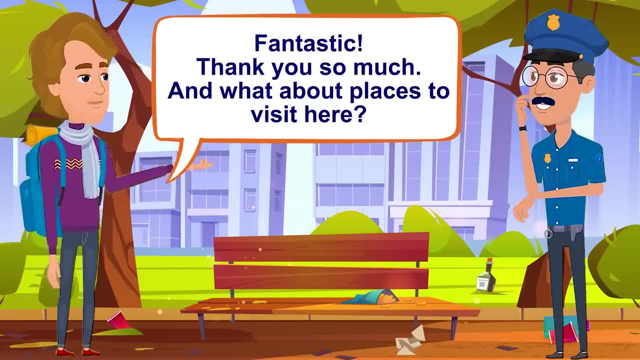 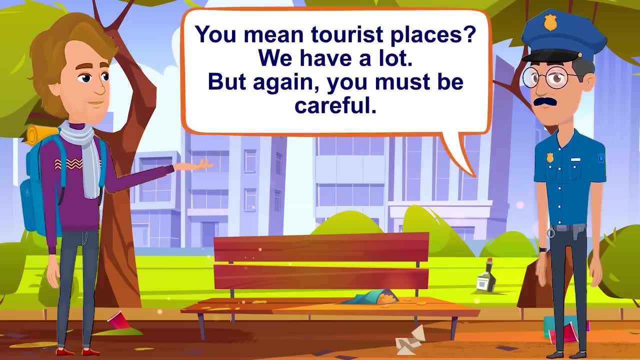 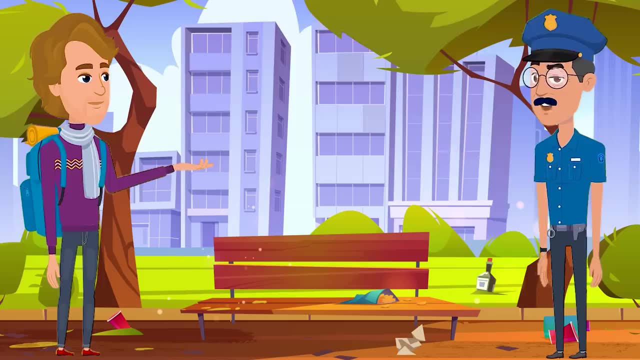 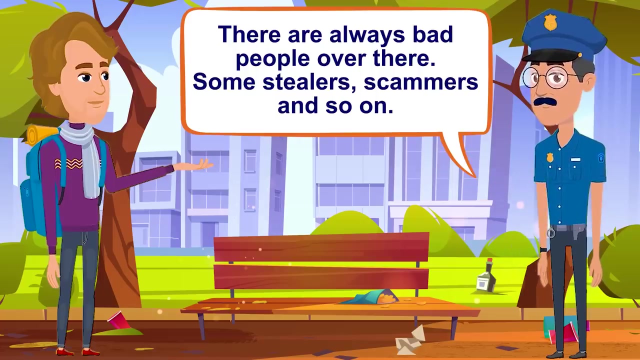 Fantastic. Thank you so much. And what about places to visit? here You mean tourist places. We have a lot, but again you must be careful. There are always bad people over there, Some stealers, scammers and so on. 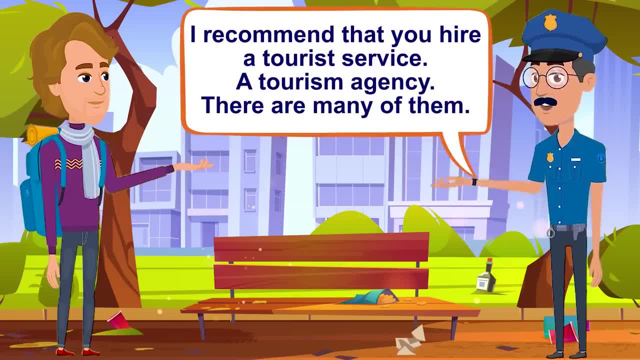 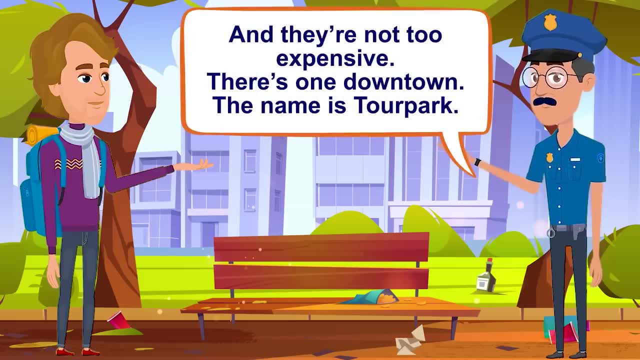 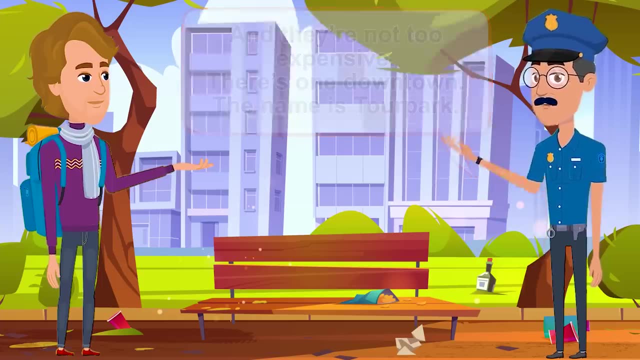 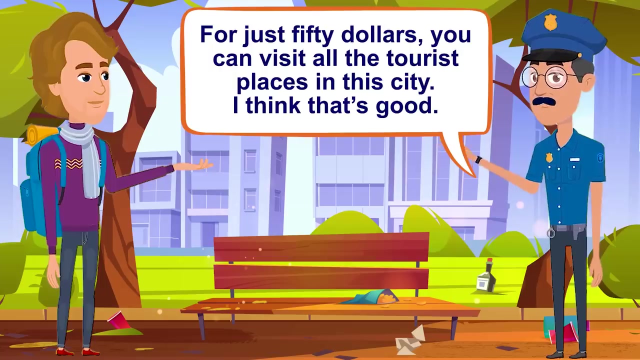 I recommend that you hire a tourist service, a tourism agency. There are many of them and they are not too expensive. There's one downtown. The name is Tour Park. For just $50, you can visit all the tourist places in this city. I think that's good. 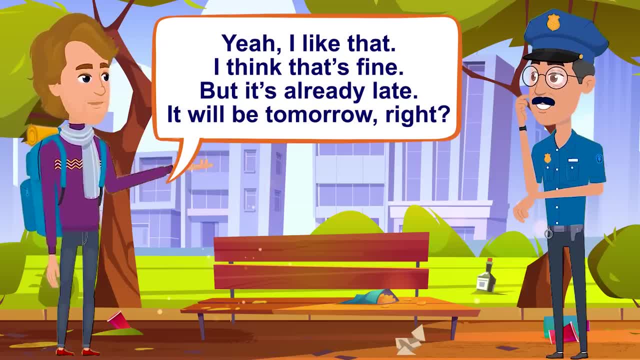 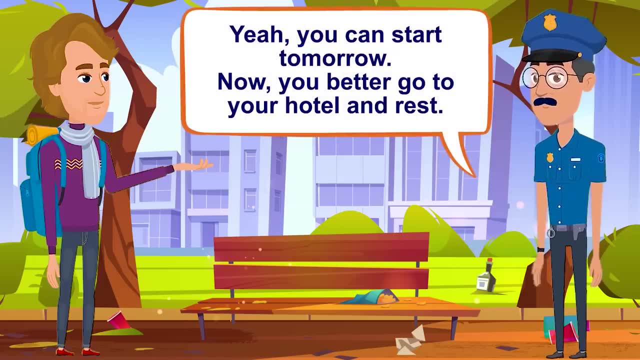 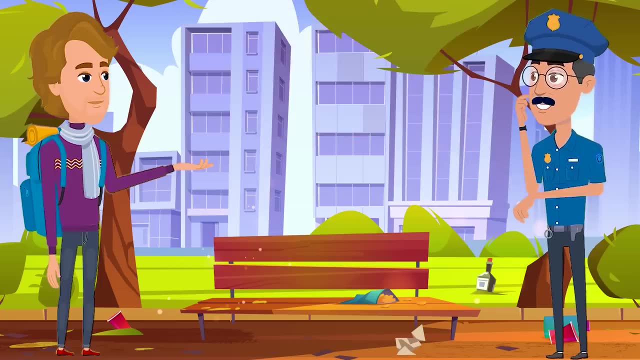 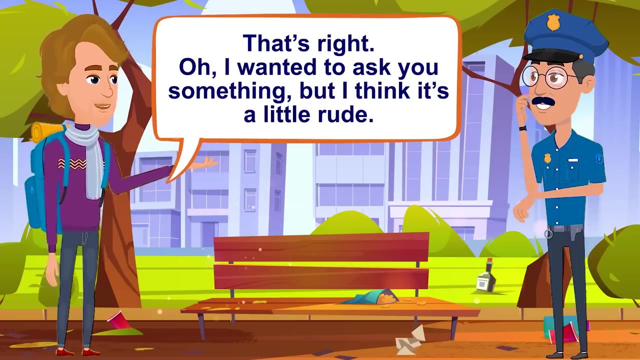 Yeah, I like that. I think that's fine, But it's already late. It will be tomorrow, right? Yeah, you can start tomorrow. Now you better go to your hotel and rest. You won't be late, right, That's right. Oh, I wanted to ask you something, but I think it's a little rude. 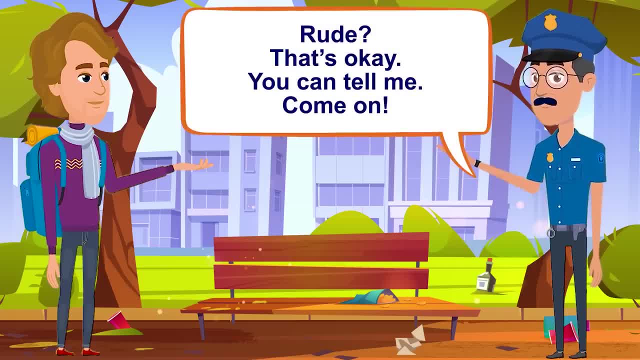 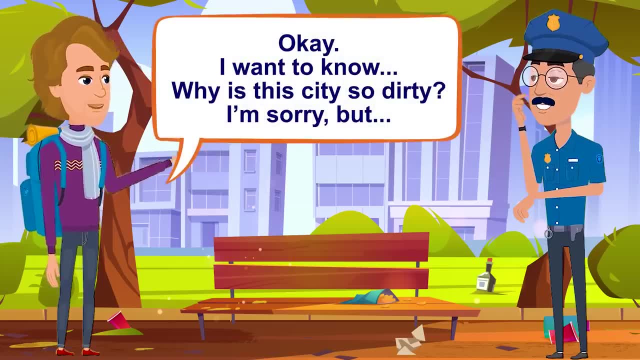 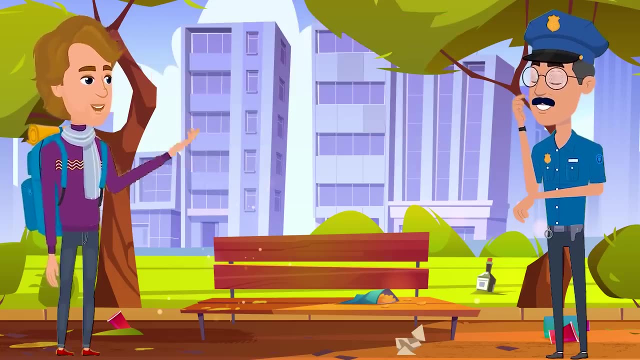 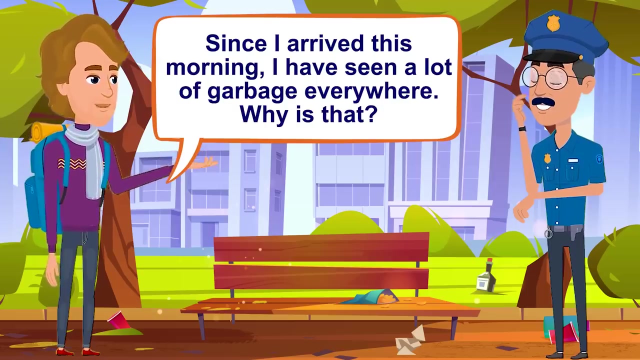 Rude, That's okay, You can tell me. Come on. Okay, I want to hear why this city is so dirty. I'm sorry, but Since I arrived this morning, I have seen a lot of garbage everywhere. Why is that? 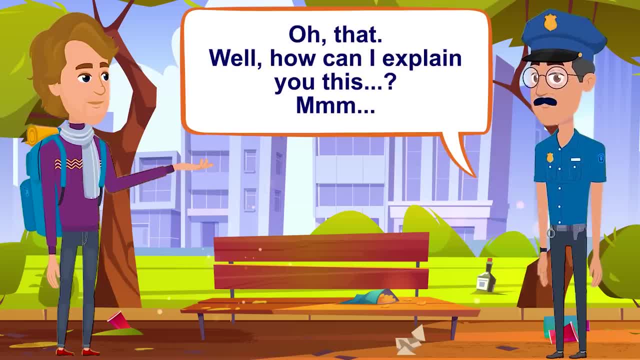 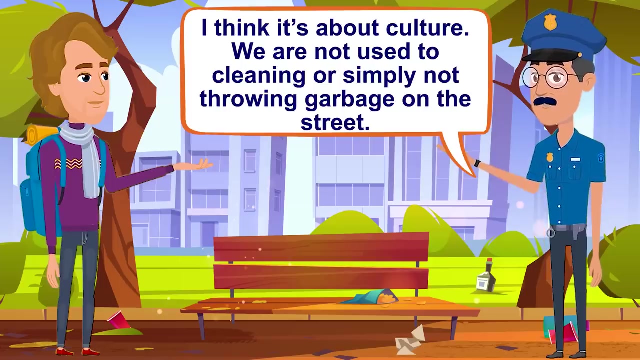 Oh that Well. how can I explain you this? Um No, I think I can't justify it. People here are not very clean people. That's it. I think it's about culture. We are not used to cleaning or simply not throwing garbage on the street. 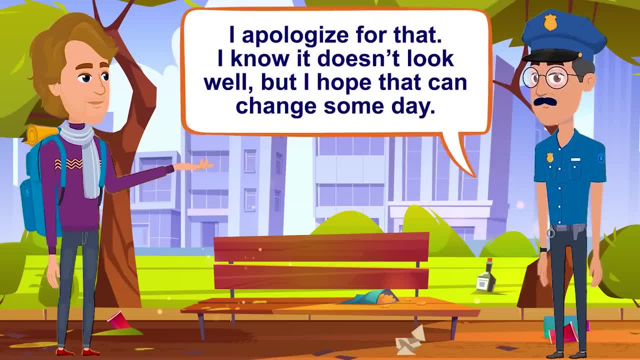 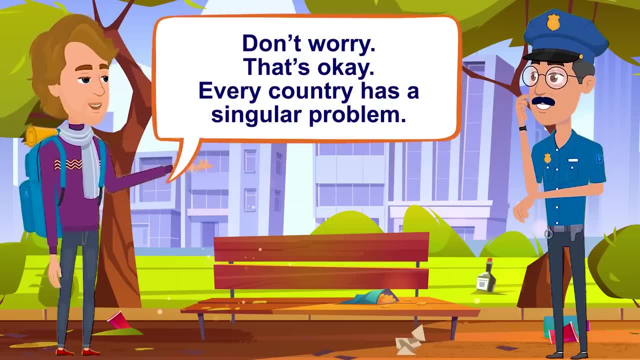 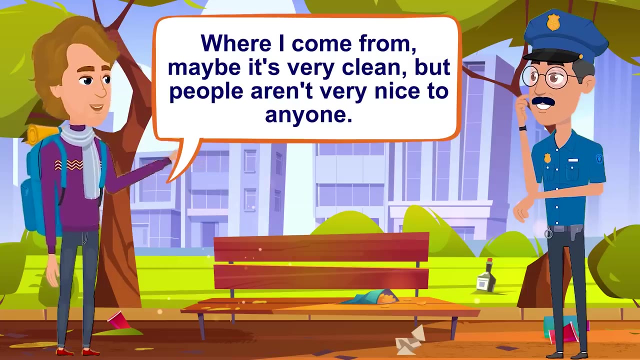 I apologize for that. I know it doesn't look well, but I hope that can change someday. Don't worry, That's okay. Every country has a singular problem. Where I come from, maybe it's very clean, but people aren't very nice to anyone. 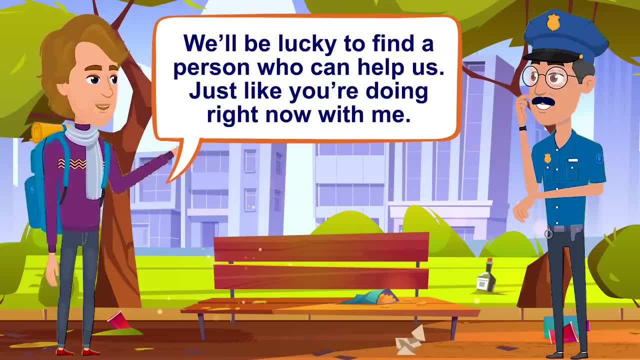 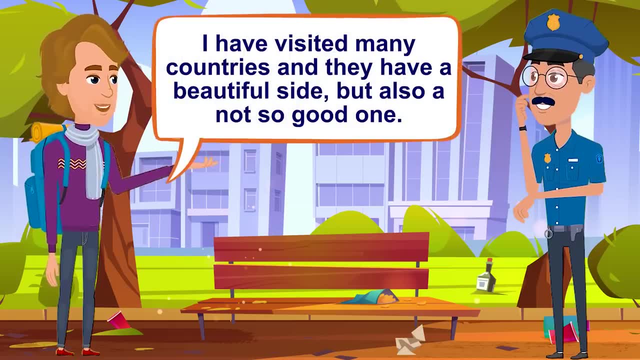 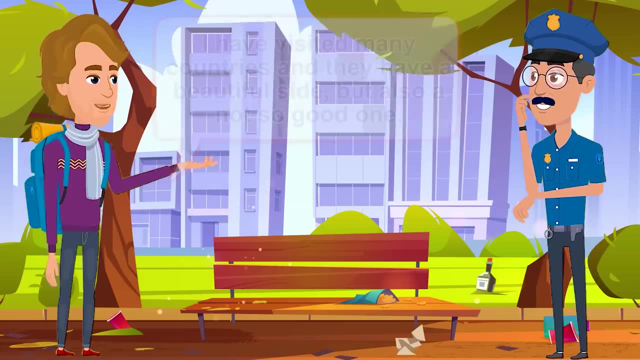 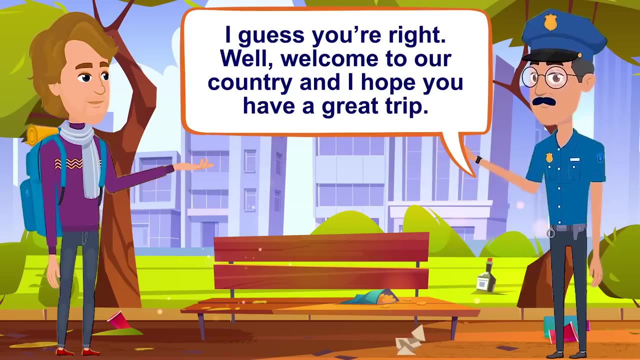 We'll be lucky to find a person who can help us, just like you're doing right now with me. I have visited many countries and they have a beautiful side, but also a not so good one. I guess you're right. Well, welcome to our country, and I hope you have a great trip. 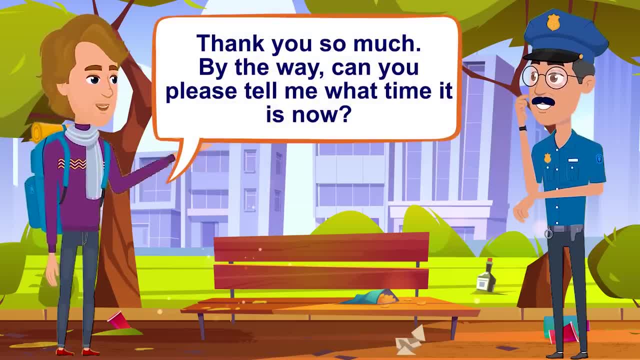 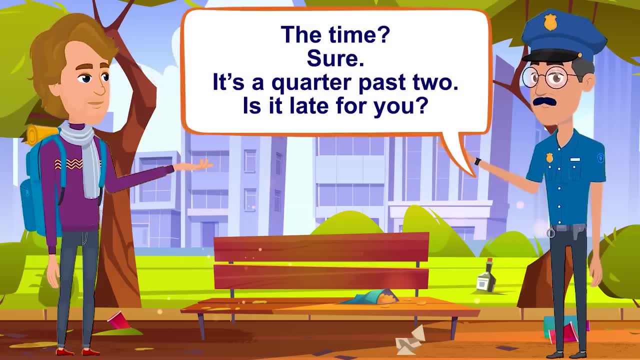 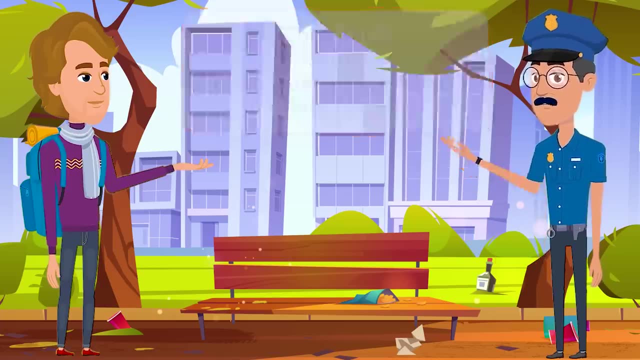 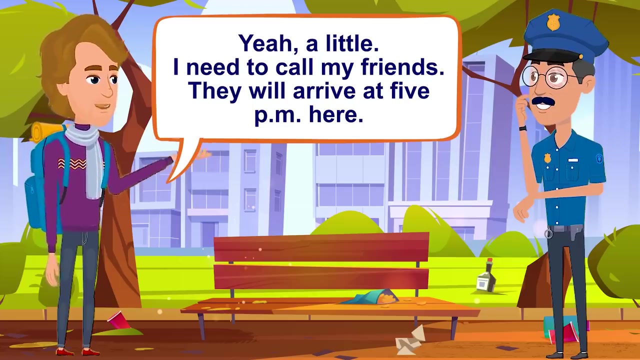 Thank you so much. By the way, can you please tell me what time it is now The time? Sure, It's a quarter past two. Is it late for you? Yeah, A little. I need to call my friends. They will arrive at five pm here. 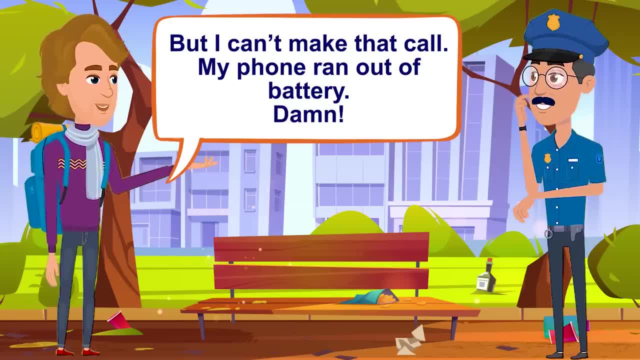 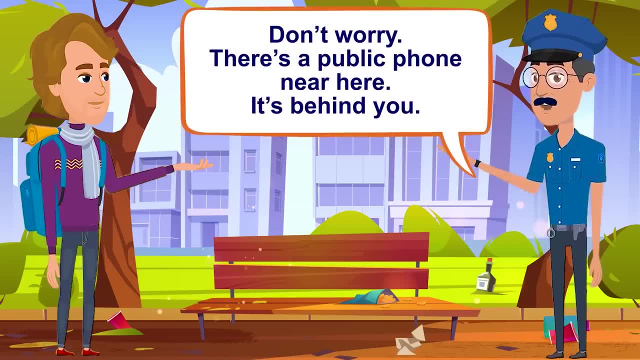 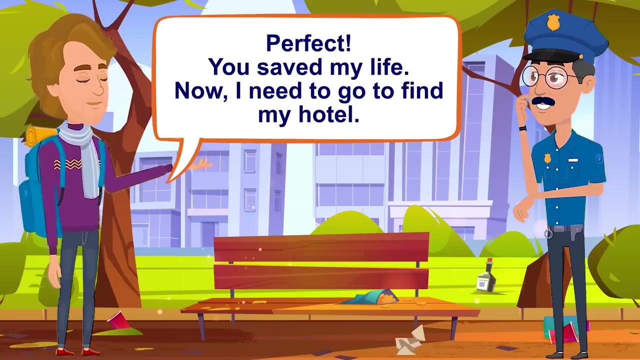 But I can't make that call. My phone ran out of battery. Damn, Don't worry, There's a public phone near here. It's behind you, Perfect, Perfect, Perfect. You saved my life. Now I need to go to find my hotel. 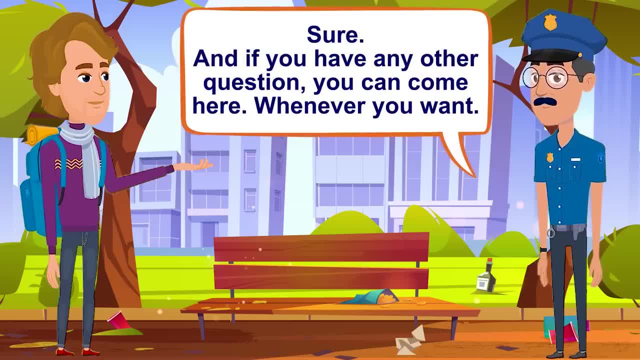 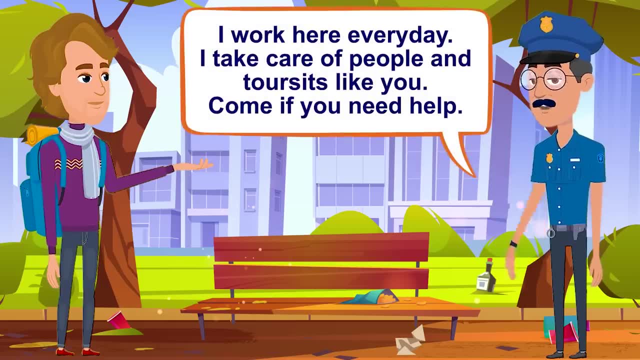 Sure, And if you have any other question, you can come here whenever you want. I work here every day. I take care of people and tourists like you. Come if you need help. That's great. Thanks, Thanks, Thanks, Thanks. 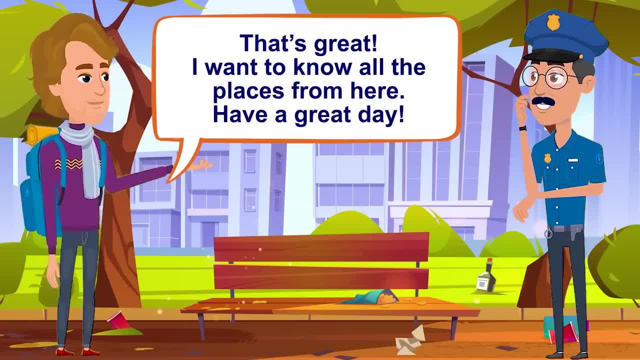 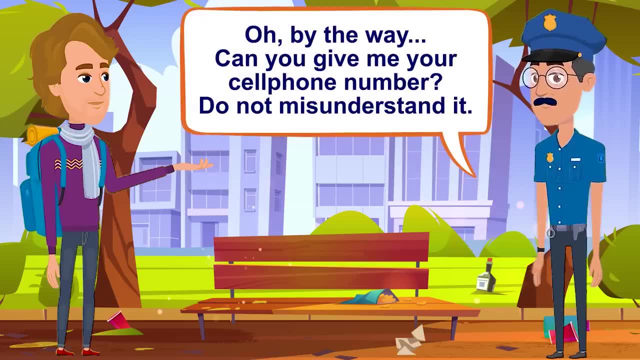